Here the main point we have to understand is that one surface glide along each other on the other surface and they form slip system. Here the main point we have to understand is that one surface glide along each other on the other surface and they form slip system. 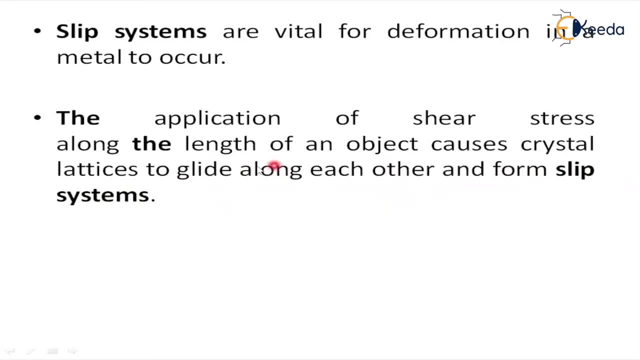 What do you mean by slip system? Is the direction is important, or the number of the slip system is important, or the number of atoms are important- All these things we are going to discuss in this slip system. Another important feature is the slip planes. are the planes with the? 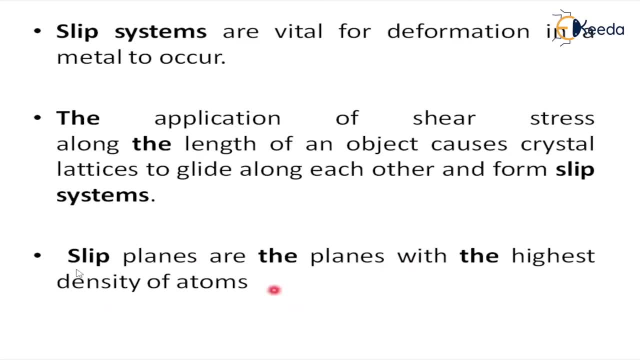 highest density of atoms. So that means the slip planes means in any structure, in any crystal structure- it may be BCC, FCC or HCP, whatever hexagonal closed packer structure- The slip planes means if the particular plane is having highest atomic density. that means 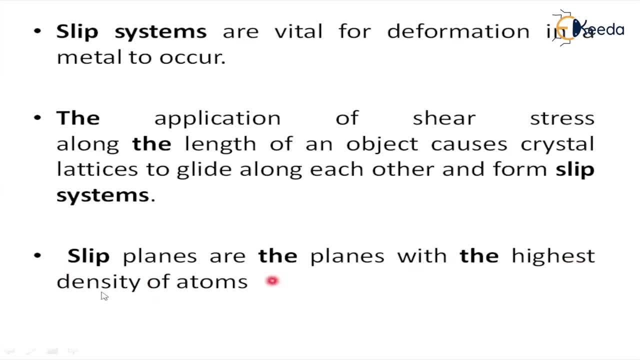 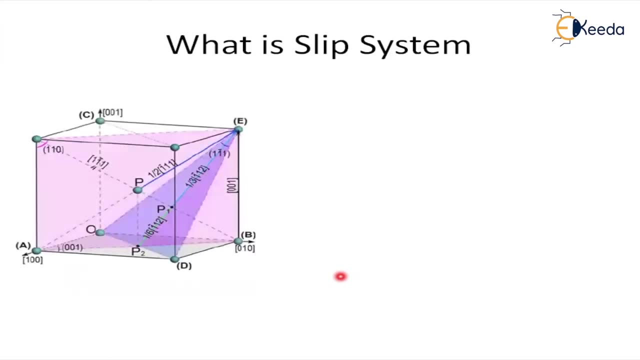 maximum number of atoms are existed in that particular plane, there is a chance to have some deformation with respect to that plane. Let us see with some images here. Here, if you observe, it is a crystal lattice. In this crystal lattice you can observe this. 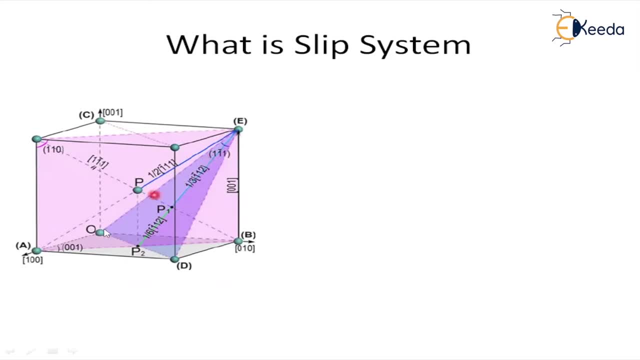 is a slip plane here. This is another slip plane. This is a slip plane. So here and here, in brackets, some numbers, they are given And this slip plane is having, or represented with some number of atoms. So this is the slip plane, So this is the slip plane. So 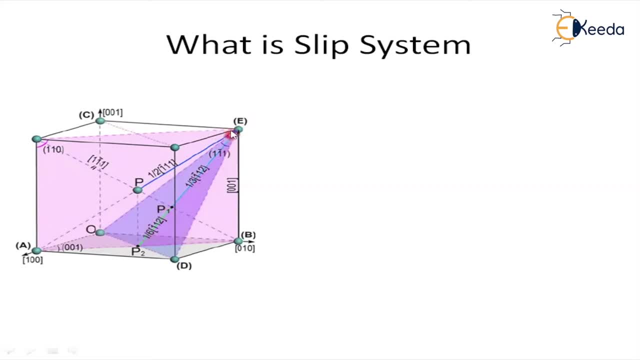 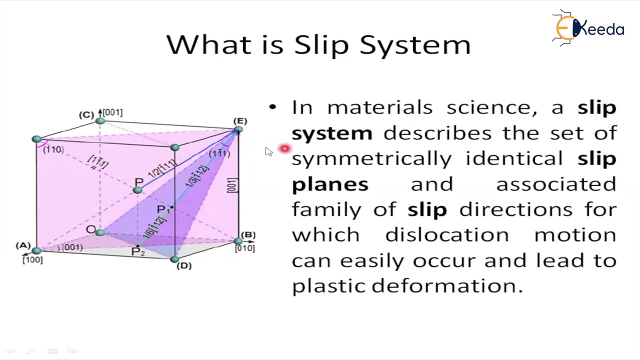 here is some number and the moment here in which direction it is moving. that is also important. before going to understand the slip direction and the slip plane, Let us have some look about. what do you mean by slip system? In material science, the slip system described the set of symmetrically identical slip planes and associated with 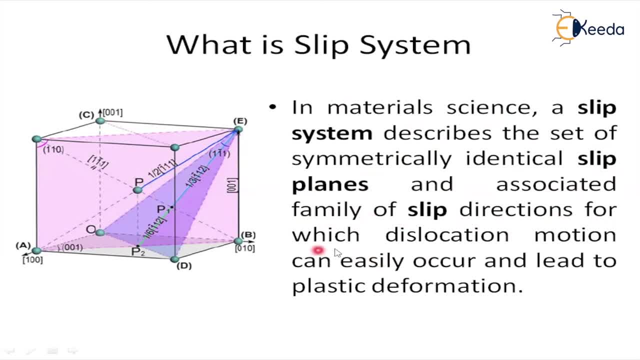 associated family of slip directions for which dislocation, motion can easily occur and lead to plastic deformation. Here the main point: if you want to observe, these slip planes lead to plastic deformation and these slip planes will move in a particular direction, only In which direction it wants to move. and what do you mean by slip plane When it? 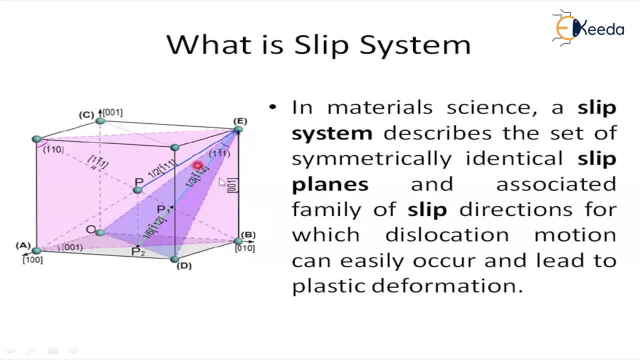 can be called as a slip plane. I already said the slip plane means the plane which is having highest number of atoms. that means atomic density. If the density of atoms are more for a particular plane, there is a chance to slip from the crystal. So that creates. 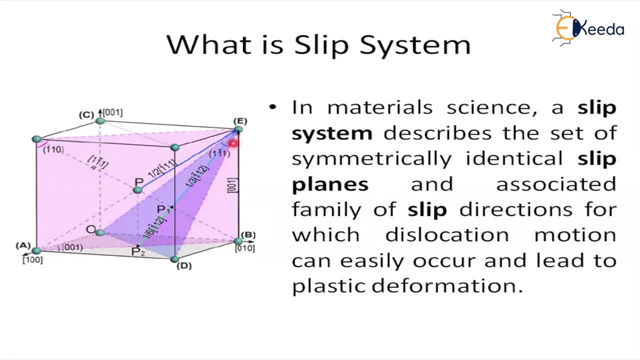 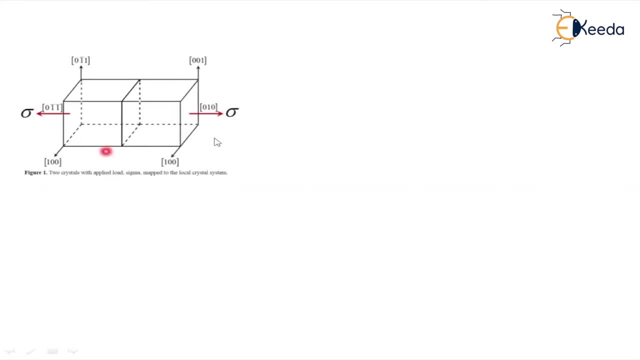 plastic deformation in the crystal lattice. Let us have some more look here. This is another picture. If you observe this picture, you can see that this is the load. here An external force is applied. If the external force is applied here, this external force makes parts of the crystal lattice glide along, each other changing. 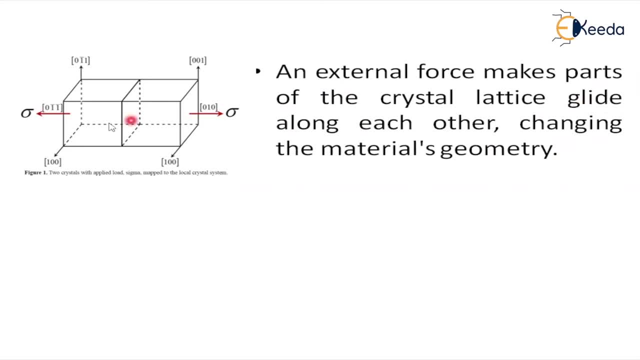 the material's geometry. This creates whatever the slip plane here. because of this slip plane the change of geometry may be observed and the main salient feature of slip system is that it depends on the material. This is the type of lattice, So that means whether it is a FCC or BCC or HCP. So depends. 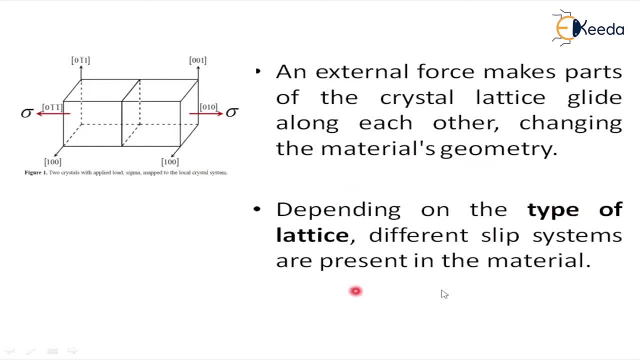 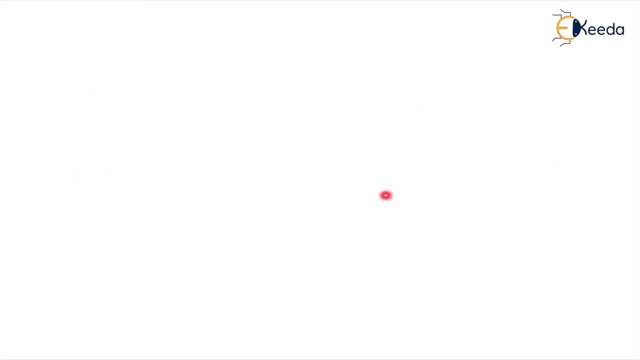 on the type of lattice, the slip system may be existed in the material. Let us have some look here. This is a closed packed plane, Hexagonal closed packed plane here. So here, when compared to other planes, this hexagonal closed packed plane more specifically slip 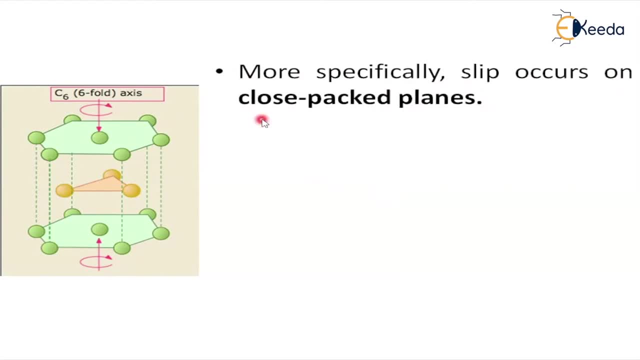 occurs on closed packed planes when compared to other means, the BCC, FCC or any other simple cubic that is. any chance of slip plane existed here, And this slip plane wants to move whenever the force is applied on the material. that means its constant force. This 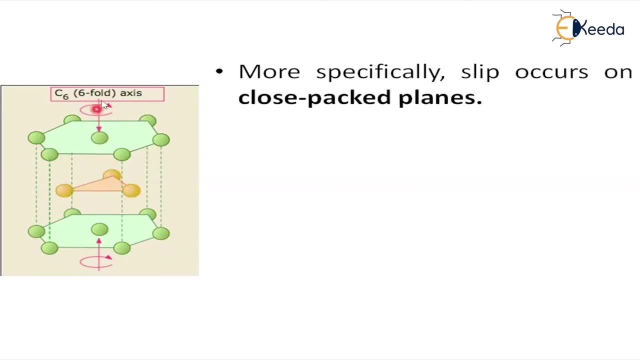 sl. physics is applied on the material while it is a closed packed plane. So le Num is material. So that means whenever the force is applied on the material, if the atomic density is existed, that means more number of atoms are existed for a particular plane. 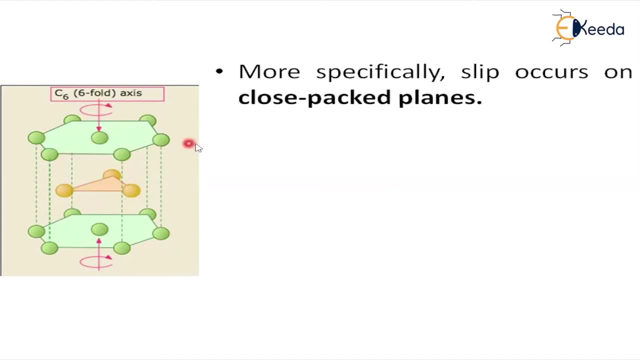 this slip or this plane may move from the crystal lattice so that the plastic deformation may be observed. This is a close packed direction here And, if you observe, the magnitude and direction of slip are represented by the Burgess vector. This Burgess vector represents how much magnitude, what is the deformation magnitude, how much it deviates, how much. 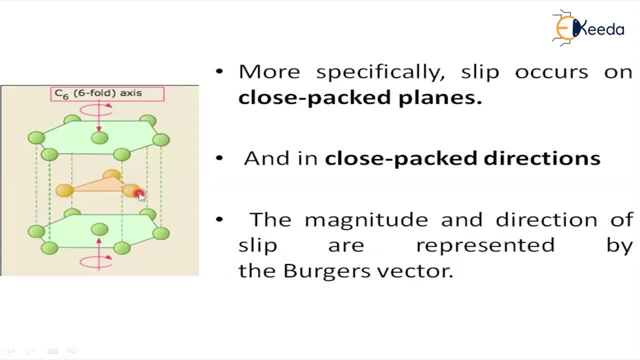 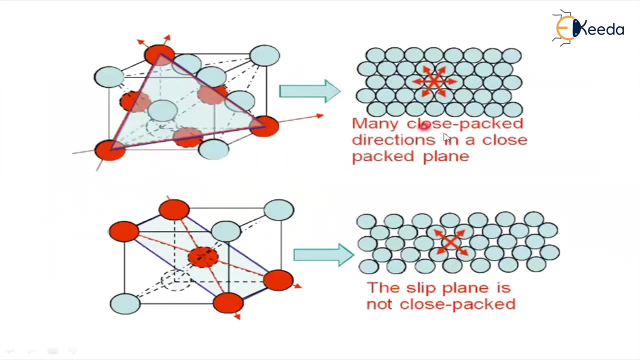 the atoms are deviated from the regular arrangement. It clearly explains the deviation or the deformation in a particular crystal lattice. Let us have some look On these pictures, Observe these two pictures here. This picture is giving a clear information. So that means it is a many close packed directions in a close packed plane. So what it means. 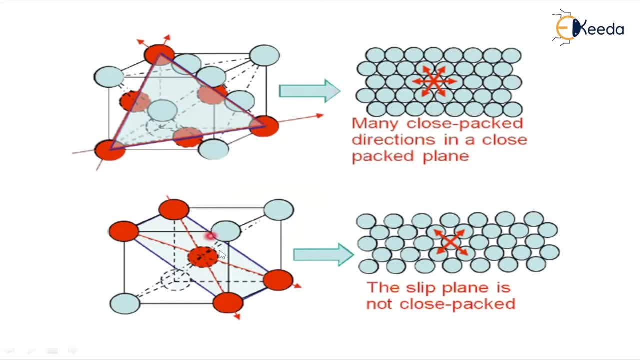 here. What is the difference between this image and this image? You can see in another form the difference between this image and this image. here, If you observe, All these atoms are close packed, but here all those atoms are, if you observe here. 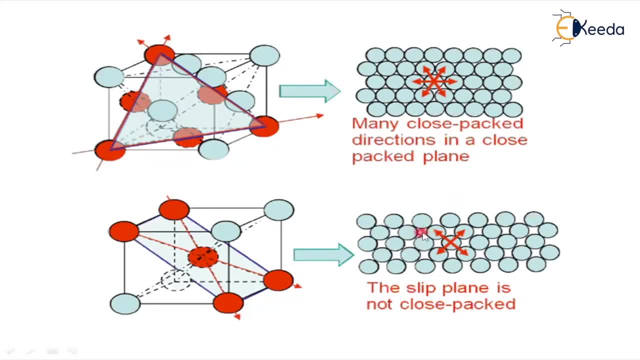 some gap is existed, some void space. This is called void space. The space between two atoms are represented as void. This is called as a void space. If the void space is existed, it is a less. there is a less chance of slip plane may be existed for a particular crystal. 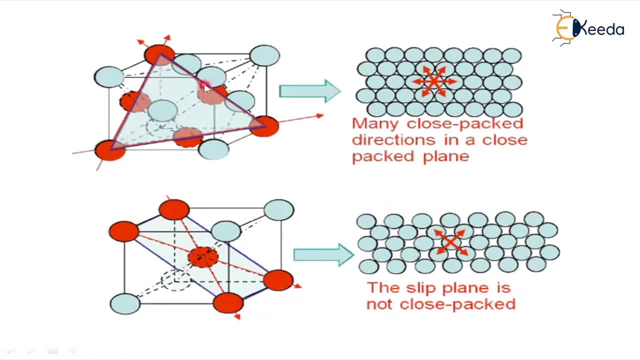 lattice On the flip side of this line here, if you observe theème here of that crystal lattice, here this specific, restricted spring of that crystal lattice is having maximum number of atoms. But here, compared to this, there is a lesser number of atoms. So that means when: 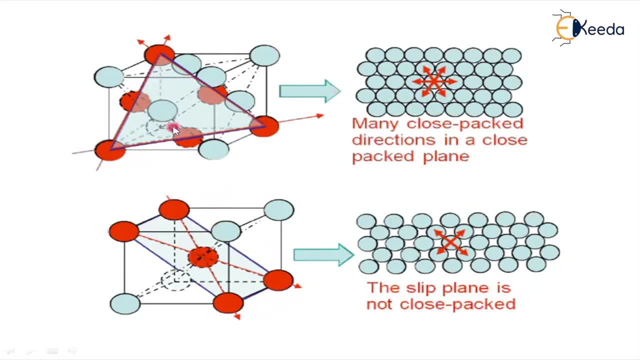 load is applied on the material. there is every chance in this inward ordering of thatциple and in the interior or the outside applications. Thus the possible지만 these slip plane might move or not. This subscribe: this is a slip plane. This is not possible from the owner audiences. 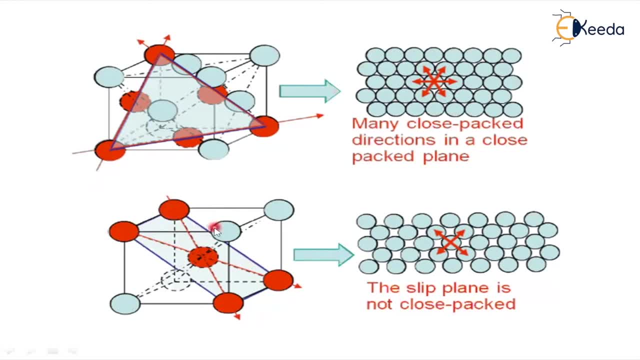 All three. It is just this. This is what we have perceived: something very letters as bar, including from the crystal plane, when load is applied because of the void spaces existed in the crystal lattice. That is the main reason in any crystal structure, So that's why the slip. 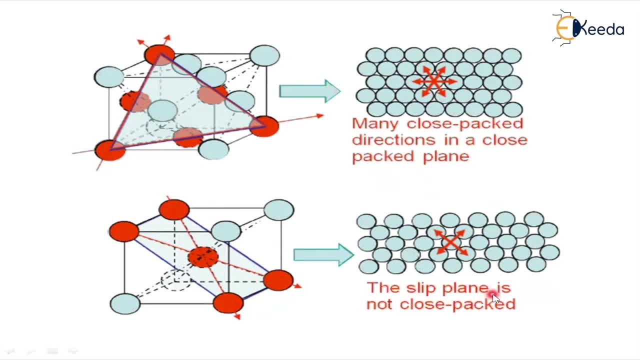 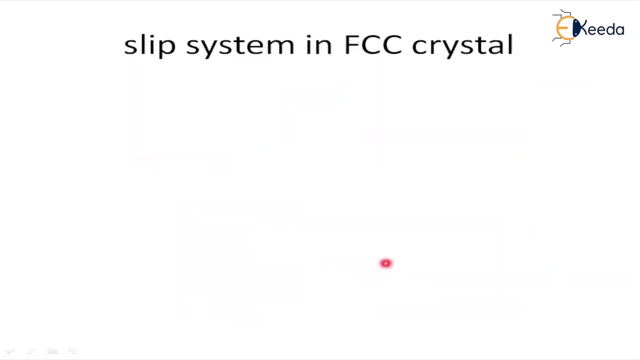 plane is completely depends on type of lattice, whether it is a FCC, HCP or BCC. If you observe the slip system in FCC crystal, So this is an FCC crystal here. This is the most favorable slip plane. That is 111 plane and the direction is 110.. That means three directions are available. 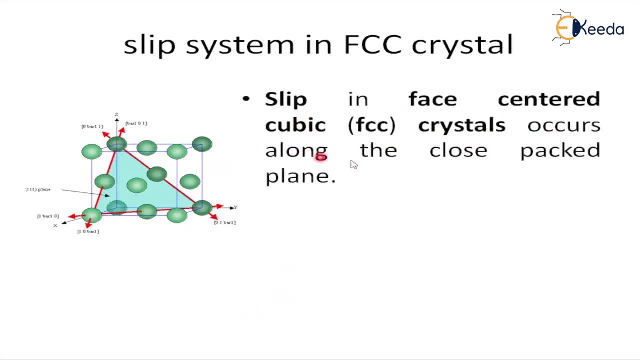 So slip in phase centered cubic crystals occurs along the closed packet plane. So this plane is having compared to other. Suppose if you take this, or if you take this slip plane, compare to all other slip planes in FCC. this 111 is having maximum number, maximum chance. 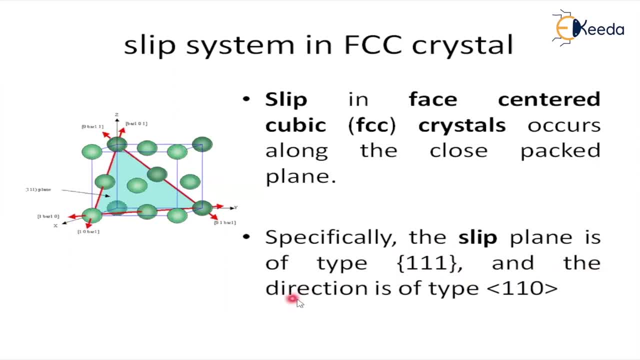 to move from the crystal lattice. in the direction The direction is also specified, direction only 110.. 110 is the specified direction. So that means in FCC crystal the slip plane is of type 111.. 1 1- 1. this is the type of the slip plane and the direction is of type 1 1- 0. this arrow represents 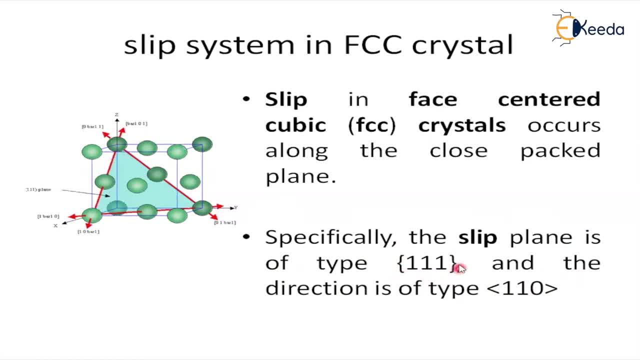 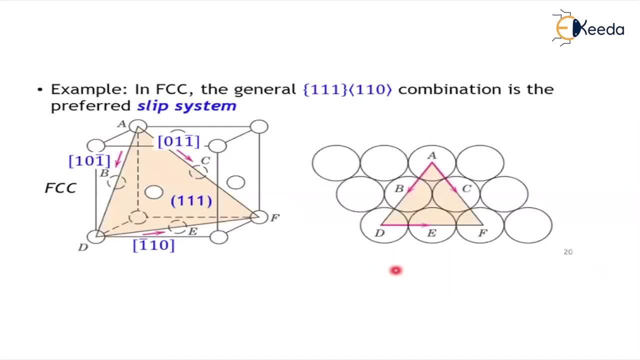 the direction. this arrow represents the slip plane number. that is a miller indices. let us have some more images here. this is another view of fcc. crystal and slip system means together, that is, 1, 1. 1. the slip plane and the slip direction together is called as slip system. here in fcc this combination is preferred one, if you observe here. 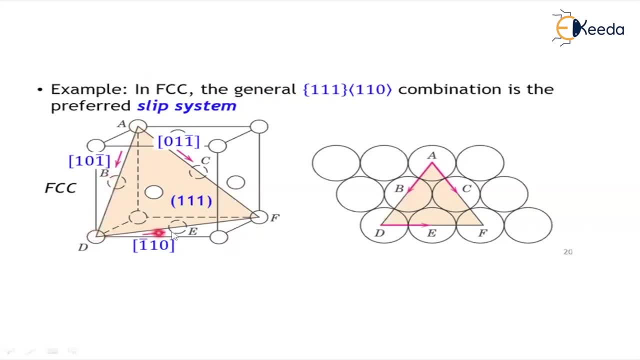 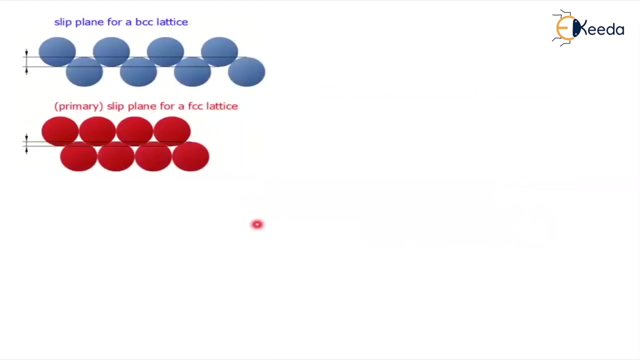 a, b, d, e, f, c and a. so this is a slip plane in which the maximum number of atoms are attached. this, that means atomic density is more. we already said that if the atomic density is more, there is an every chance to move this plane from the crystal lattice. let us have some more. look here. 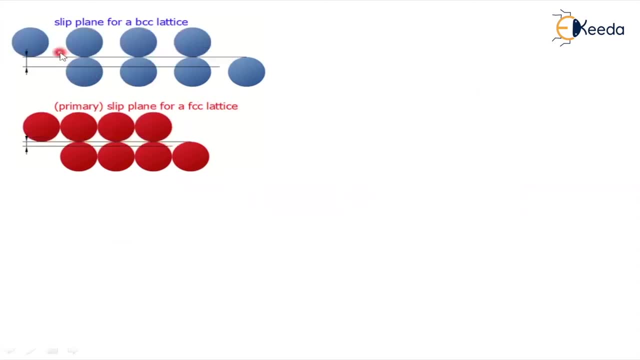 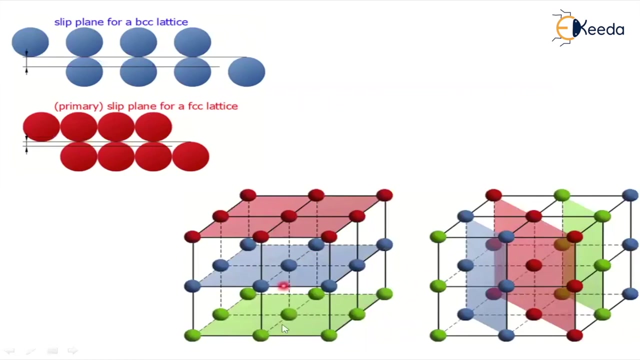 this is the representation in BCC. there exists a gap. if you observe FCC, the gap is not existed here. this is another representation. different type of slip planes, or existed here? all these colors, pink color, blue color, all these colors in different directions. so in all these slip planes, only few slip planes. 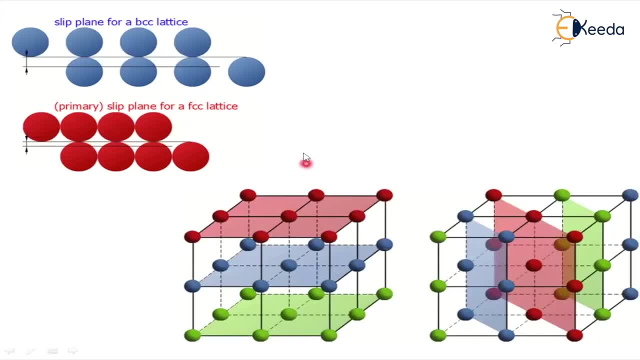 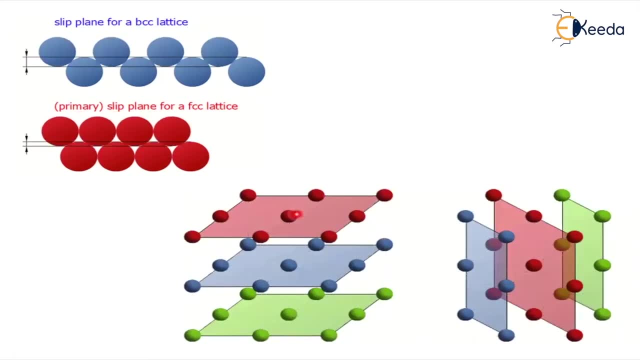 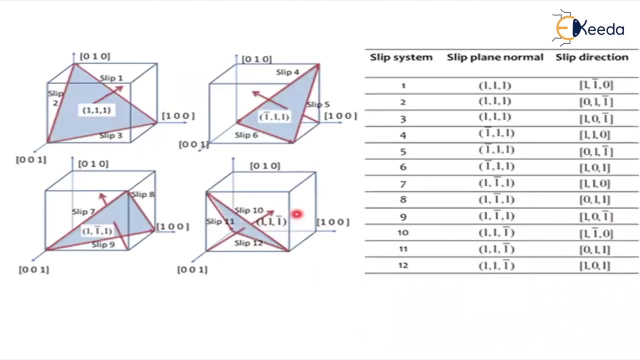 may move from the crystal lattice when load is applied on the material. let us see what are the various planes which moves from the crystal lattice when load is applied in a FCC structure. so these are the four images which clearly shows which plane moves from the crystal lattice when load is applied. if you 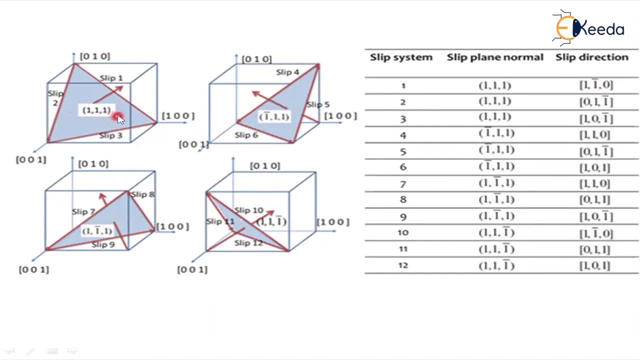 observe, this is one one. one is a one slip plane in three different directions. this is one bar one one. this is in another direction. this is another direction. this is another direction. all these planes move in different directions. so, totally, 12 slip systems are existed. all these 12 systems are the. 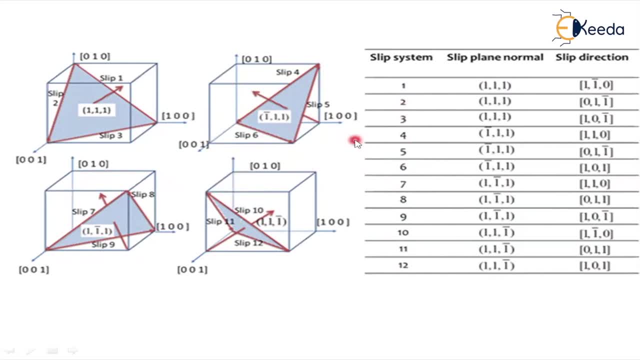 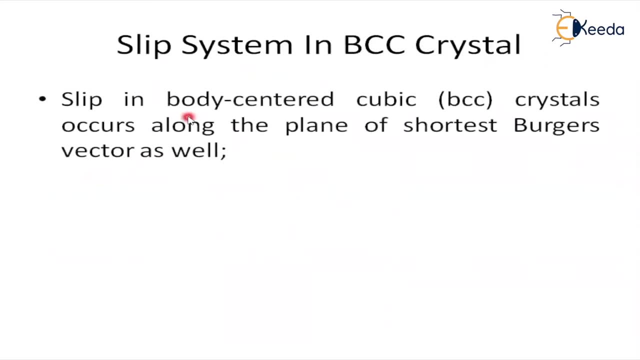 favorable directions for FCC. If you observe the BCC, that is, the slip system in BCC, if you observe the slip in body centered cubic crystals occurs along the plane of shortest Burgess vector as well And the main salient feature is compared to FCC, FCC is not having 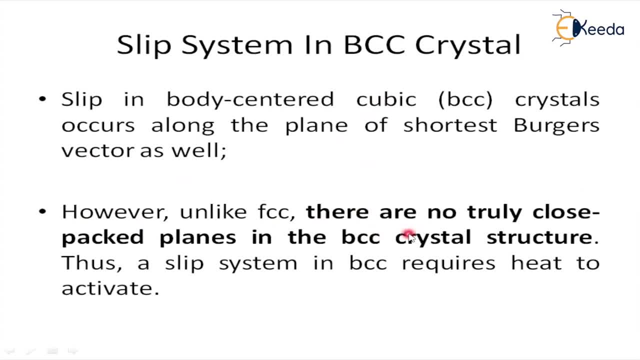 that much packed number of atoms. So that means atomic density is very less. There are no truly close packed planes in the BCC crystal structure. Thus this slip system- there is a slip system in BCC- requires heat to activate. So that means some heat is required, some. 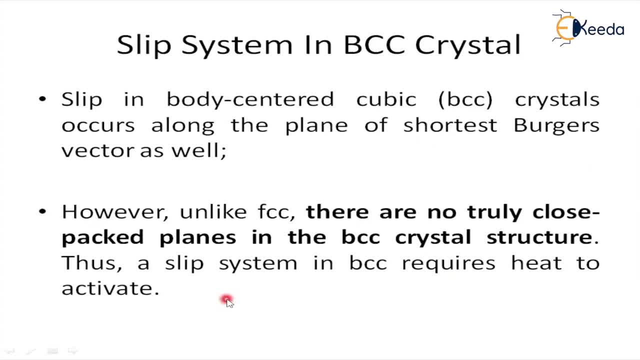 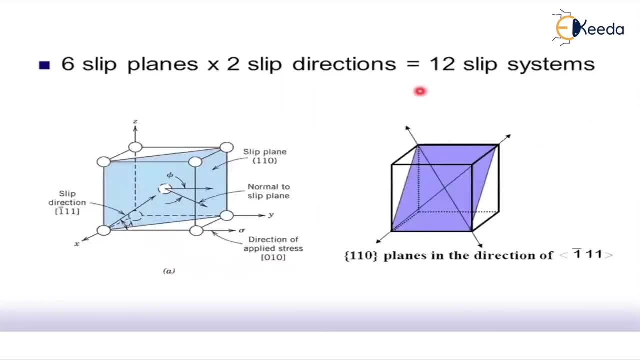 temperature is required to generate slip in body centered cubic structure. Let us have some look. How many number of slips may be existed in body centered cubic structure? If you observe this crystal lattice, there is a center atom, this is a body centered atom and this is a. 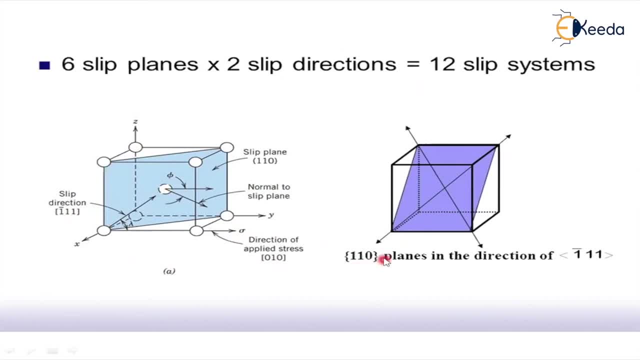 body centered cubic structure. So here this is 110 planes. All these are 110 planes. These are favorable slip planes. Why we have taken this slip plane? Because this slip plane is having maximum number of atoms compared to other slip planes. This is because this slip 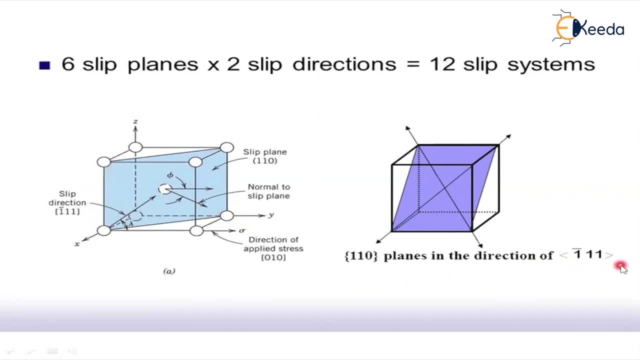 plane is having maximum number of atoms compared to other slip planes and in the direction 111.. Here you can observe these two images here. This is the first image, which clearly shows the slip plane, the most favorable slip plane in body centered cubic structure. 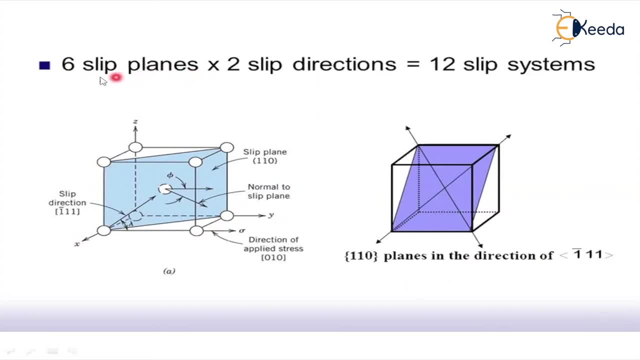 Totally these type of planes are existed in body centered are six, that is six slip planes and two slip directions. Totally 12 slip systems are existed in the body centered cubic structure. existed in body centered cubic structure. Now, the last one is the most favorable slip. 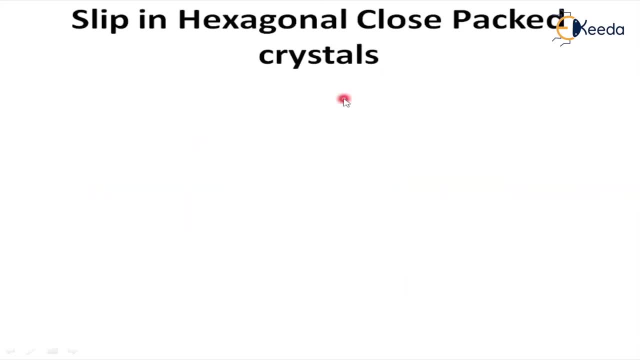 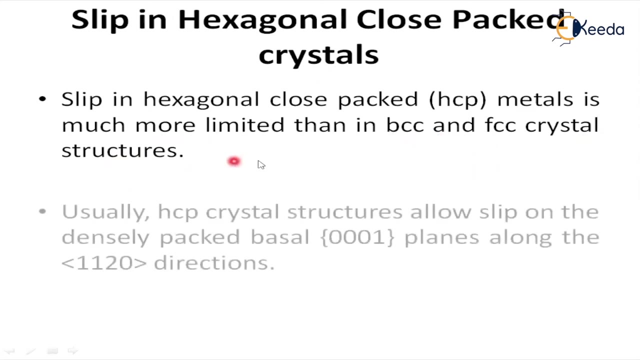 planes which are existed in hexagonal closed packed crystal is like this. If you observe the first sentence, slip in hexagonal closed packed, that is, HCP metals is much more limited than in BCC and FCC crystal structures. Usually HCP crystal structures allow slip on the body. 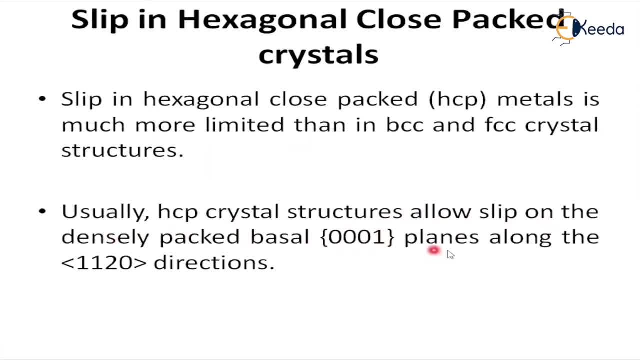 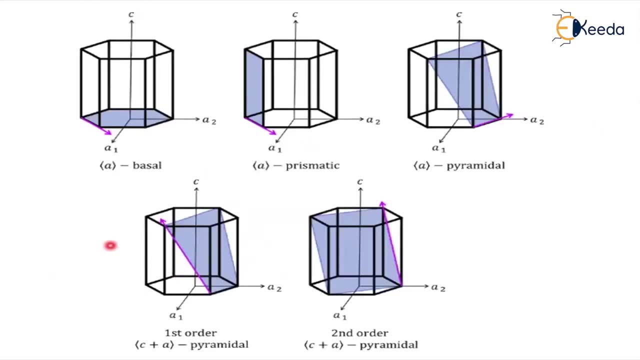 densely packed Bessel, So 0001 planes along the 1120 direction. So this is the favorable planes and these are the favorable directions Here, if you observe the hexagonal HCP crystal structure. So this is Bessel plane here. This is prismatic and this is pyramidal and this 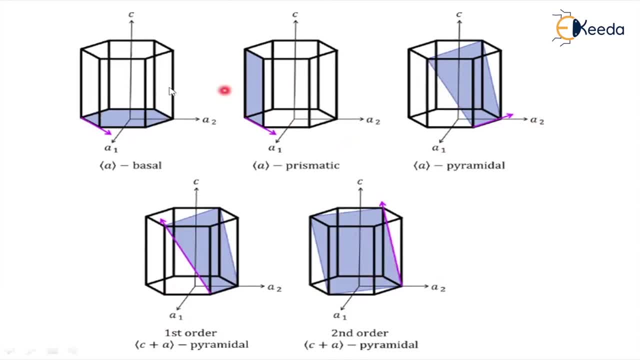 is another pyramidal and this is another pyramidal. All these are favorable, hexagonal, closed packed slip planes. So here, when compared to BCC and FCC structure, HCP structure is having maximum number of slip planes. Why? What is the reason behind this? Why, Because these slip planes. that is this. 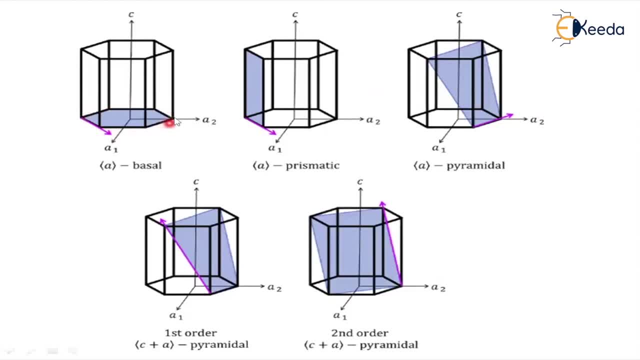 HCP is having maximum number of atomic density. So that's why if the maximum number of atoms are existed for a particular area or in a particular area, then there is every chance to move that particular plane. from the crystal lattice You can clearly observe the slip.